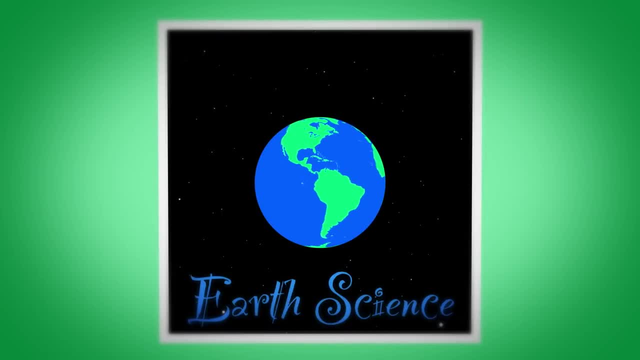 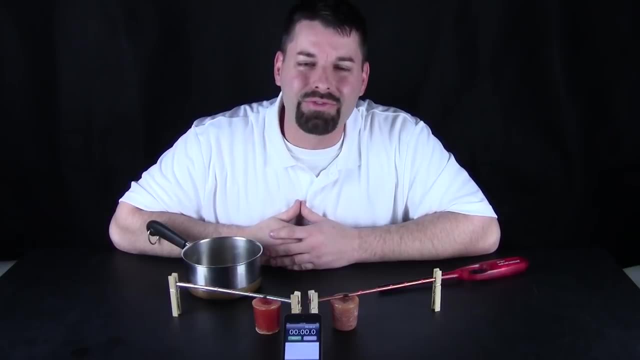 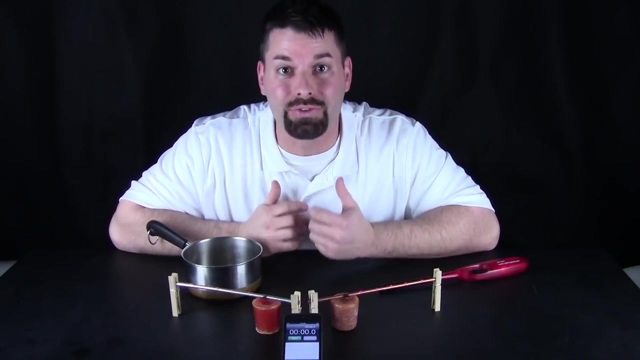 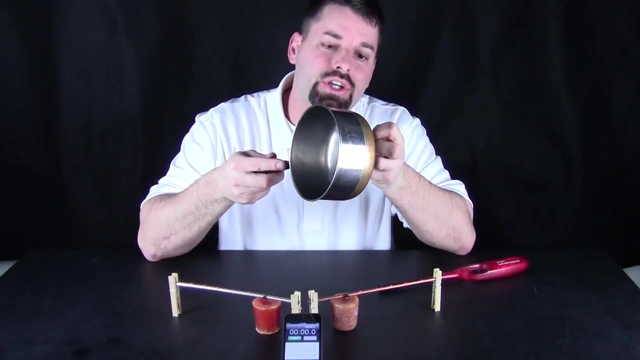 Hi, I am Jared. Welcome to Fun Science Demos. The big idea today is that different types of matter allow heat energy to move through them at different speeds. Take a look at this pot. What is the purpose of the pot? It heats things up. Heat energy travels through it. 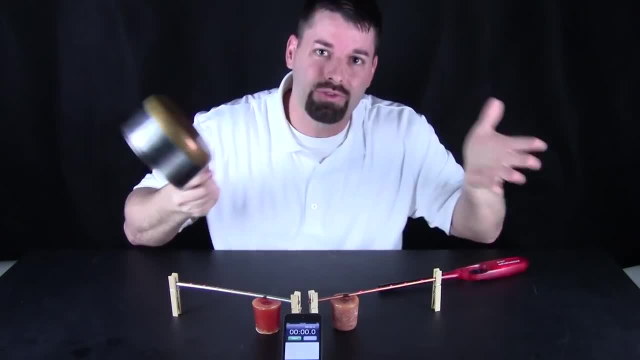 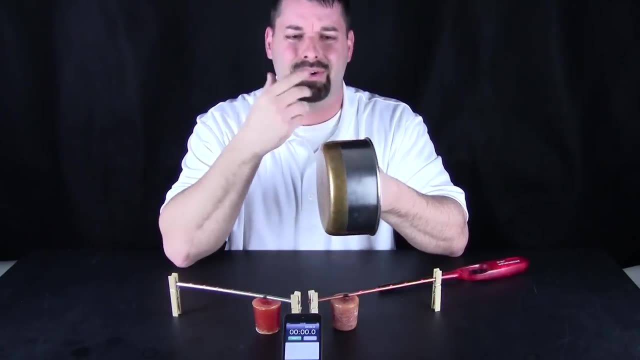 I said, different types of matter allows heat energy to move through them at different speeds. This pot has two different types of matter. The top part is steel and the bottom part is copper. Why is the copper on the bottom? Why not reverse it? It sounds like I need. 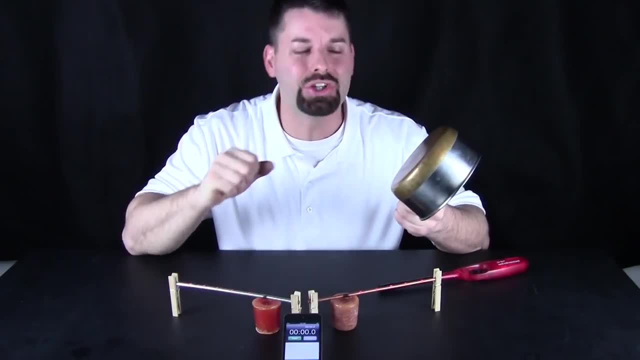 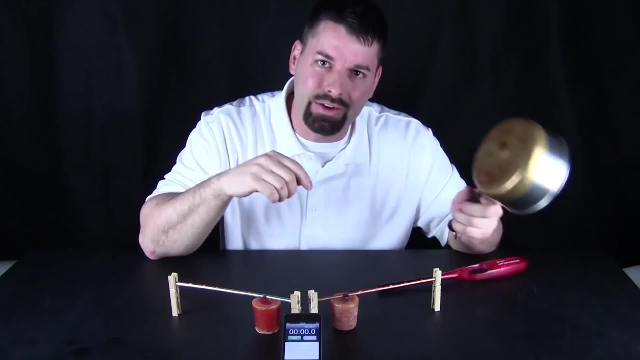 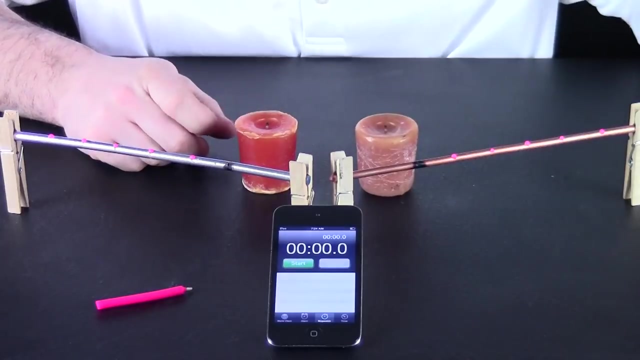 science to answer that question. Now, I cannot see heat energy moving through matter. I cannot see the heat energy moving through this pan. Using science, we can show you how quickly that heat energy moves using this demonstration. I have two candles that are going to provide our heat energy And we have our two different. 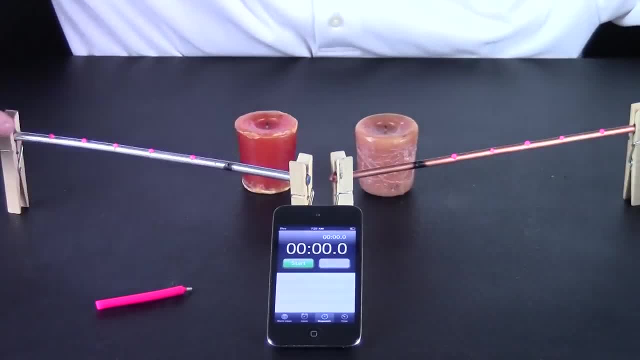 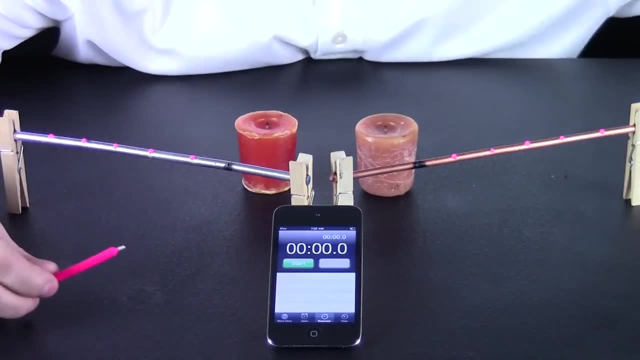 types of matter. We have a copper rod and a steel rod. Clothes pins are our little stand. We have our timer, But what are these pink dots? Well, we needed something to show you the heat energy moving down the rods. So we took wax from a birthday candle and put little 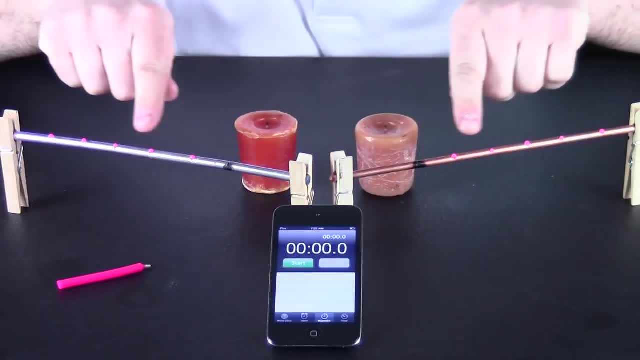 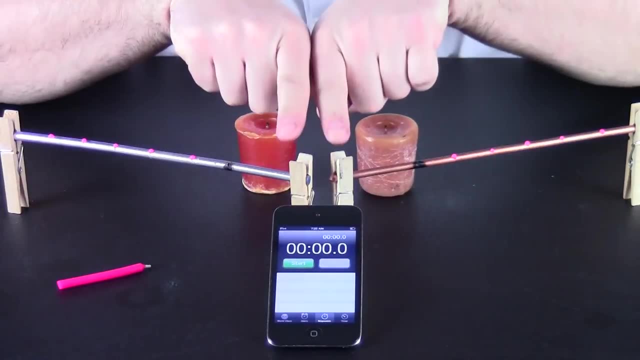 drips along our rod. As the heat energy moves down the rods, it melts the wax And we should be able to see the heat energy moving down the rod. Let us see how quickly that heat energy is moving down each rod. Is it moving more quickly? 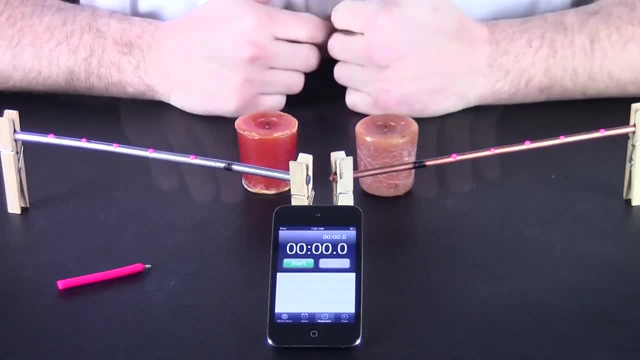 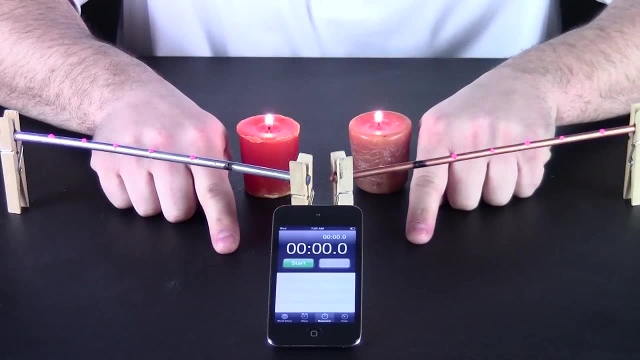 down this rod? Or is it moving more quickly down this rod? Let us take a look. Our candles are lit and we are ready for our race to begin. I am going to slide these candles under our rods providing the heat energy, And I want you to watch carefully to see how quickly. 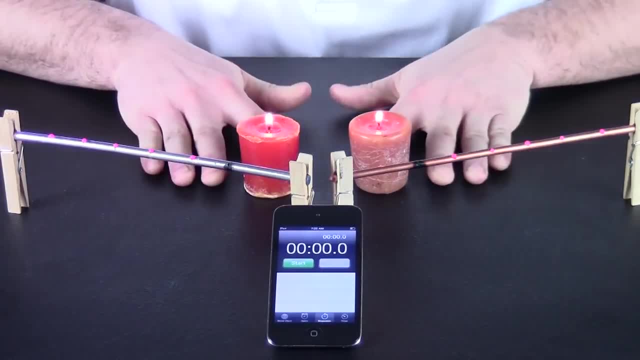 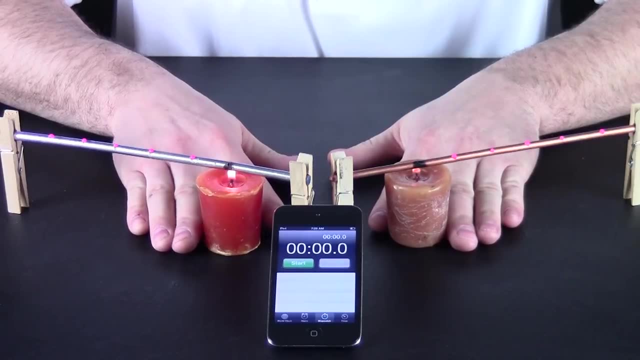 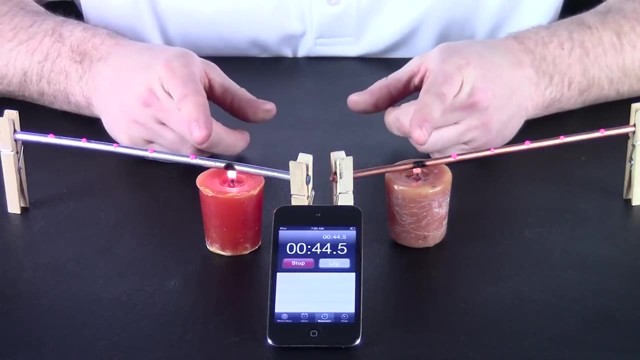 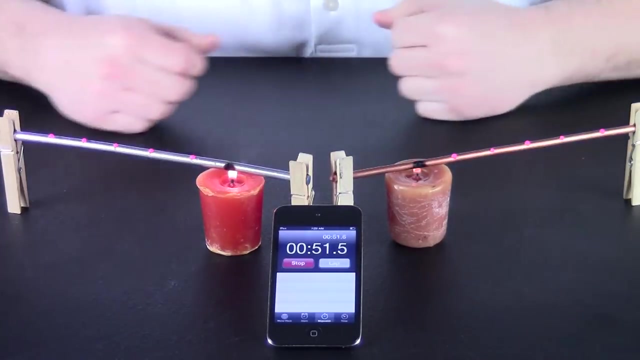 that heat energy is moving down the rods. Once I slide the candles under, we will start the clock and the race begins. Here we go. So the flames are starting to provide heat energy, And that heat energy wants to move. It wants to move down to our rods And it does not look like anything is happening. 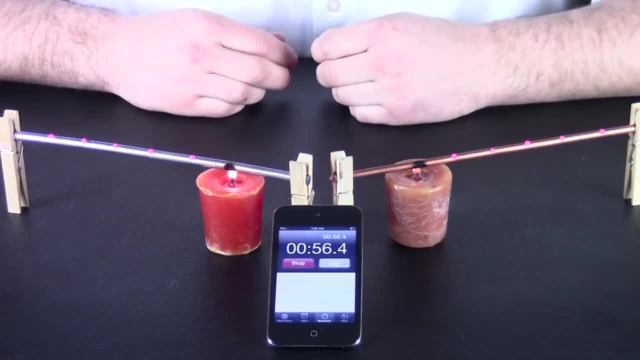 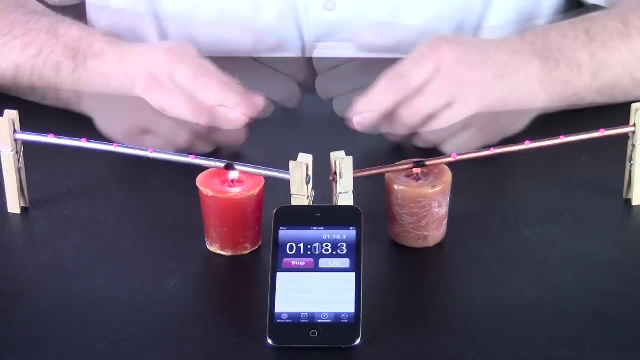 It does not look too exciting at all, Because you cannot see it, But once that heat energy gets to these first two drops, they are going to start to melt. Let us see. 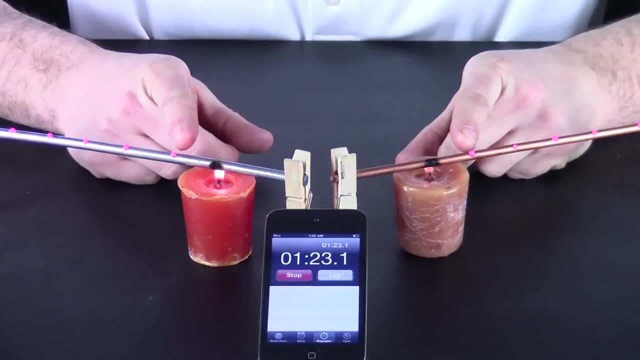 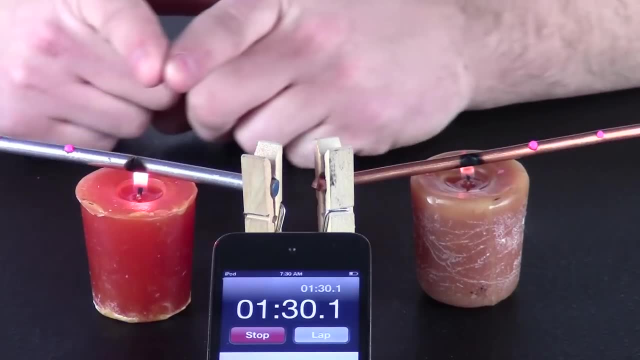 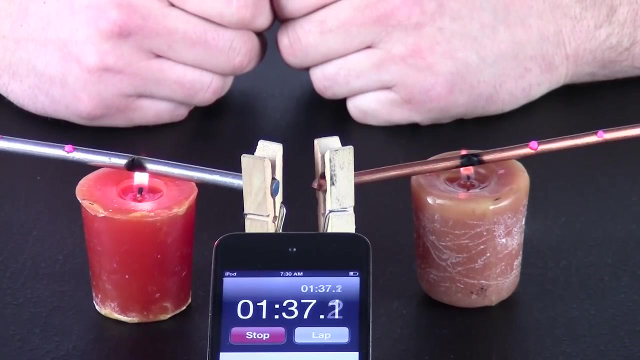 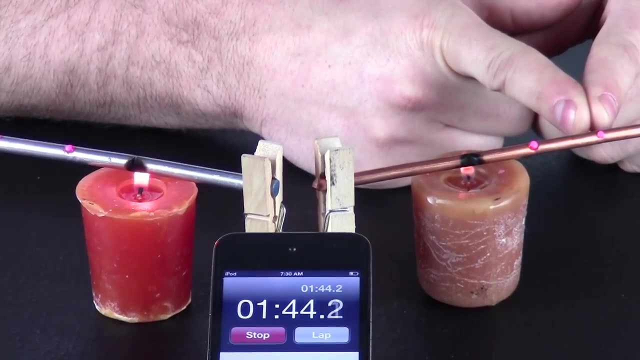 look very carefully at each of these dots, you will see the bottom starting to melt. on each one It looks like the copper is melting a little bit more than the steel. Uh oh, If I look carefully at the copper I can almost see the second, the second dot of wax starting. 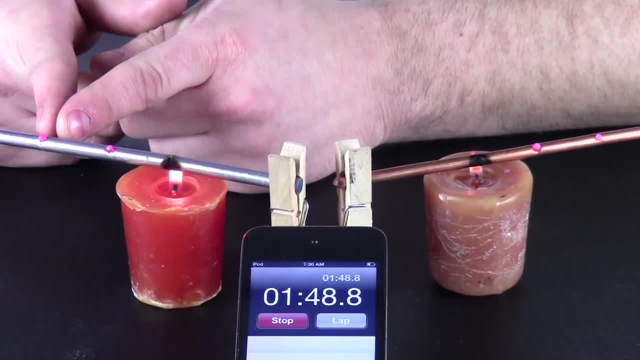 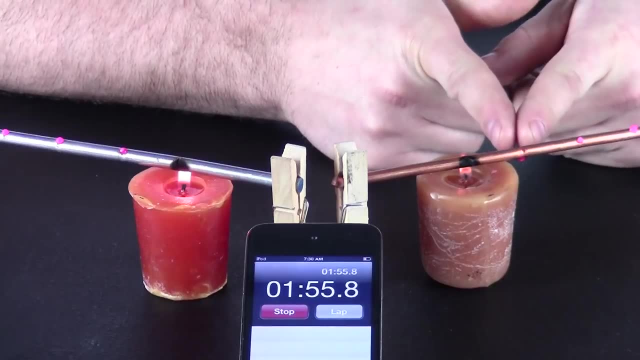 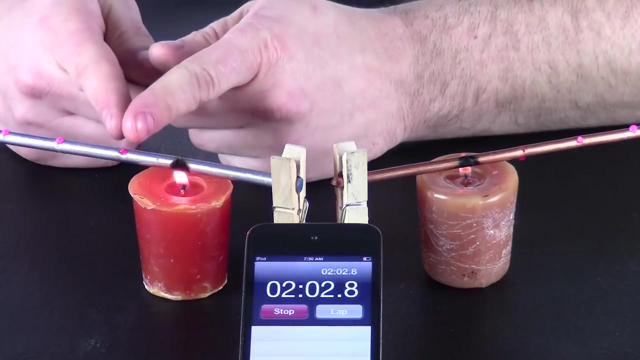 to melt a little bit. Nothing is happening on my steel dot. Both dots are starting to melt. That means the heat energy's travel. oh, the copper went down first. Wait a second. it must mean the heat energy's moving a little more quickly through the copper. This is starting. 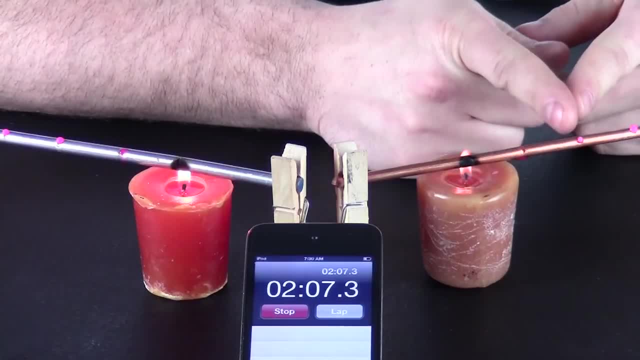 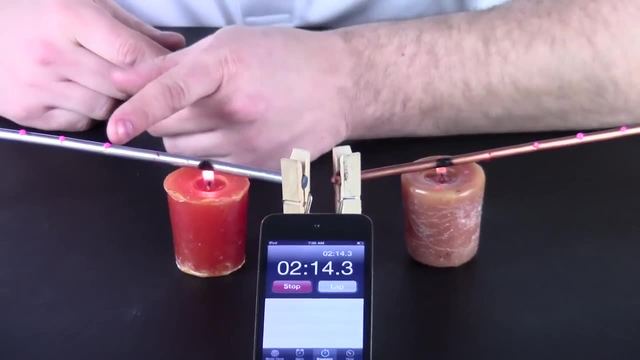 to melt. now the race is heating up. The second dot on the copper is starting to melt. it's almost ready to go. I have the first dot on my steel that's melted, but the second dot begins to melt and I'm getting a little separated and I don't want to start the process a-. 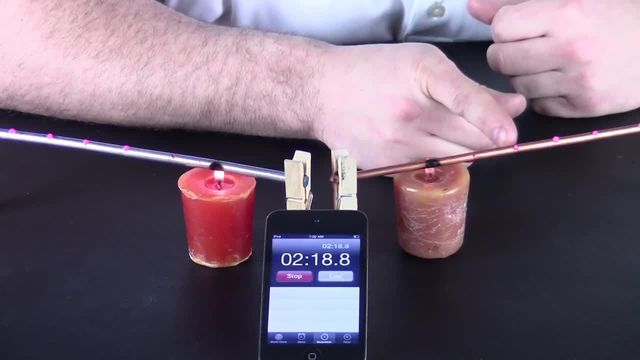 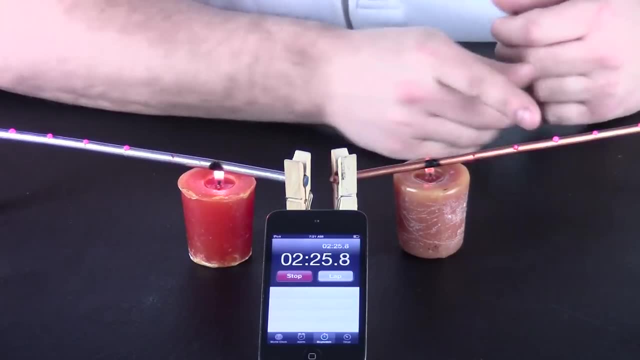 not melting at all. I can really see this dot starting to melt. Wait, my third dot is starting to melt on my copper. That heat energy is moving more quickly down this copper. I can see it with my eyes. Take a look at our second dot on the steel. No melting, It is. 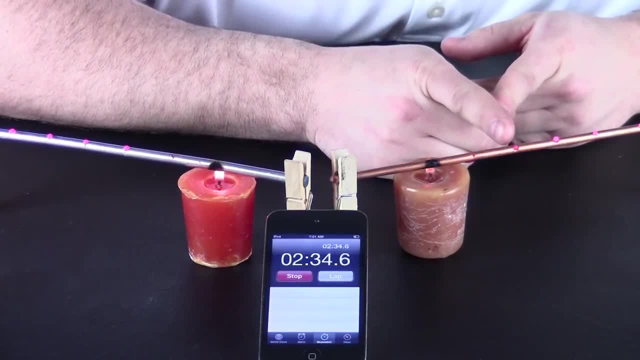 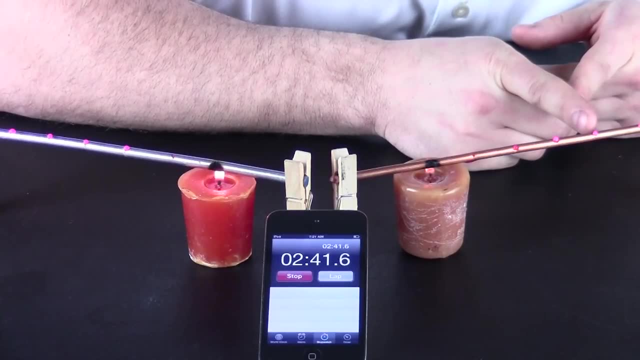 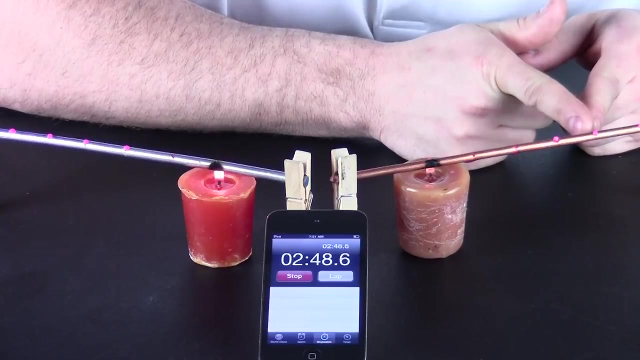 moving more slowly. The second dot on the copper is ready to go. Oh wow, Take a look, I move over. The fourth dot on the copper is actually starting to melt. now We have one, two, three, four dots on the copper starting to melt. Only one dot on the steel, The second. 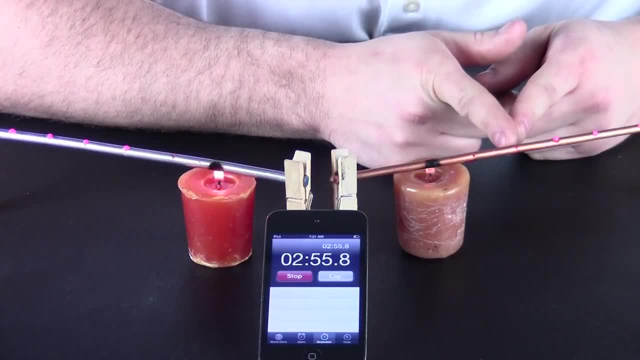 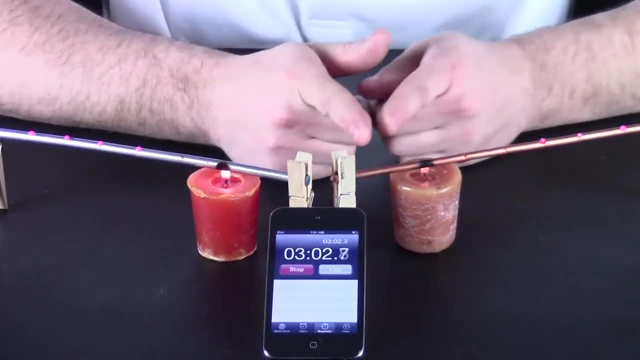 dot has not even started to melt. The second dot: look at the dot on the copper. It is down. My third dot on the copper is ready to melt. Fourth dot: My fifth dot is starting to melt on the copper. We can see the heat energy moving down the copper. It is not even 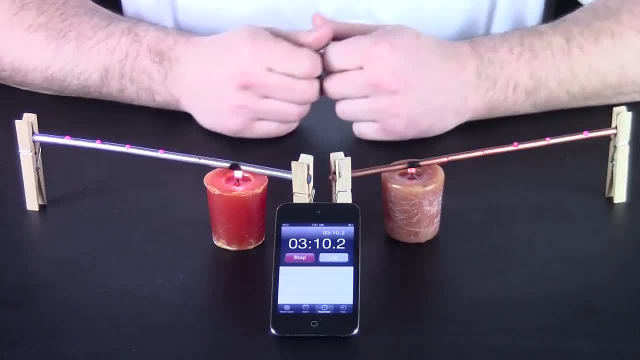 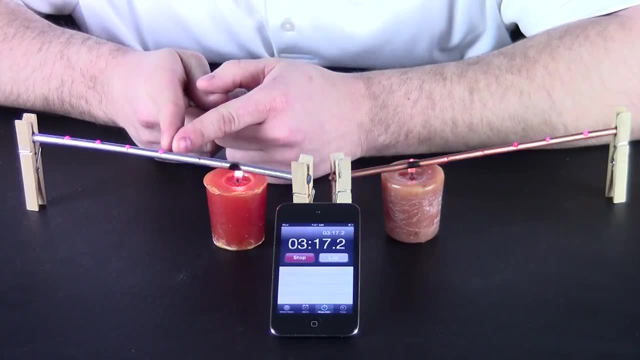 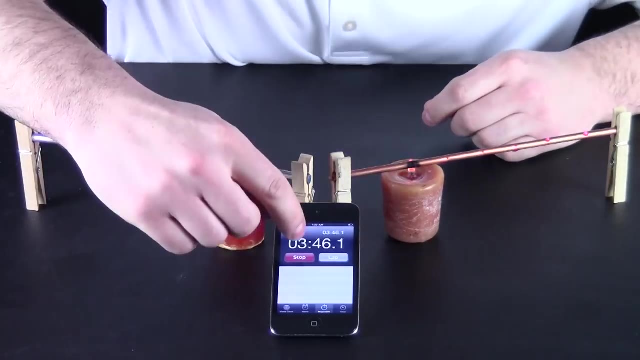 moving down the steel. Well, it is, but it is moving slowly. We are at three minutes and I am almost melting my third dot. My second dot has not even started to melt on my steel. The third dot is getting ready to go. Oh, it goes down. Let us hit.